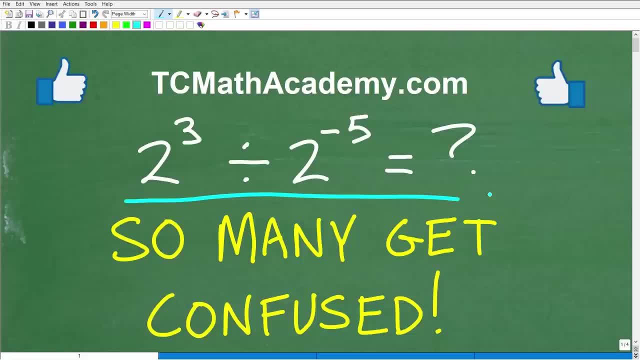 Like algebra. But before we get started, let me quickly introduce myself. My name is John. I have been teaching middle and high school math for decades. It really is my true passion to try to make learning math as easy as possible. So if you need assistance in mathematics, check out my math help program at TCMathAcademycom. You can find a link to that in the description below. And if this video helps you out, don't forget to like and subscribe, as that definitely helps me out. 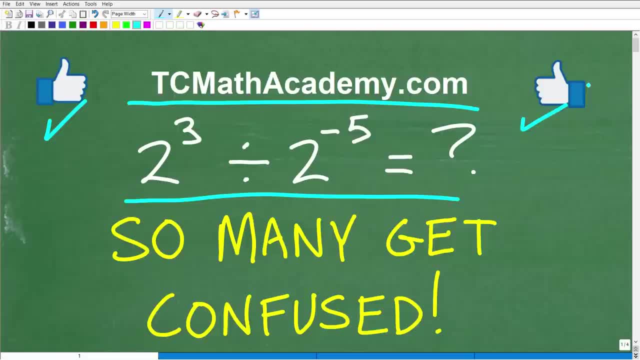 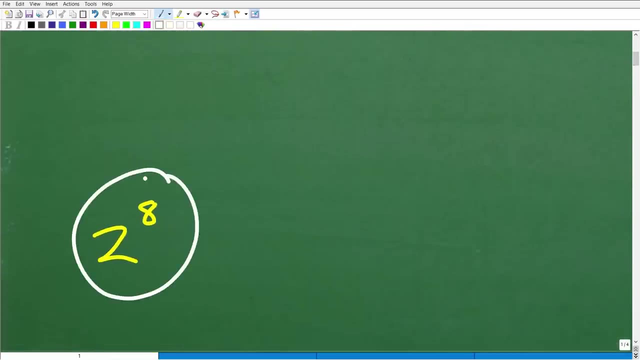 Okay, again, we want to put our calculators away. So, two to the third, divided by two to the negative fifth power, What is this equal to? Well, we're going to express our final answer here in terms of a power. So here it is. It's two to the eighth power. Now, of course, you can go and be like: okay, two to the eighth power, That's two times itself. Eight times, That's a lot of multiplication, So you don't need to do that. If you did that, that's great, But the answer that I'm looking for is two to the eighth power. 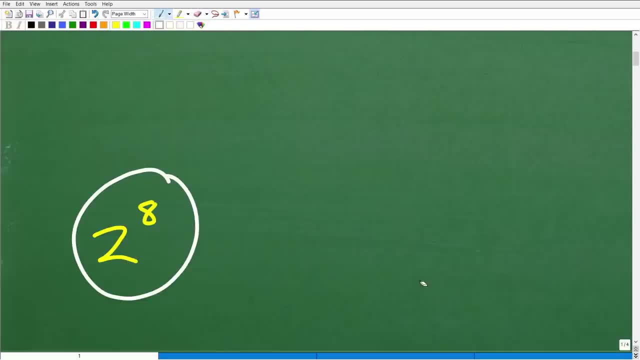 Now, when it comes to working with powers in mathematics, it's not correct If you leave your answer. let's say two to the negative. third, right, If you turn in an answer with a negative exponent, typically your teacher is not going to like that. They're going to kind of frown upon that. So you're not done working with a power until you have all your exponents as positive. Okay, so this is a pretty common 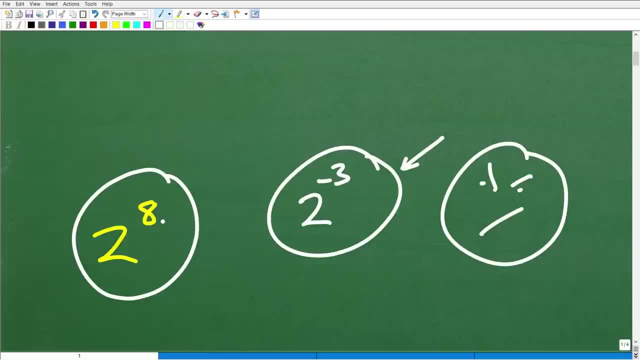 convention. Most math teachers probably would agree with me on this. So just get in the habit of not leaving your final exponents, your final powers, having negative exponents. If you don't even know what an exponent is, don't worry, I'm going to explain all this in just one second. But if you got this right, that is fantastic. Let's go ahead and celebrate by giving you a nice little happy face and a plus, a 100% and multiple stars, So you can brag to your friends and family that indeed you are. 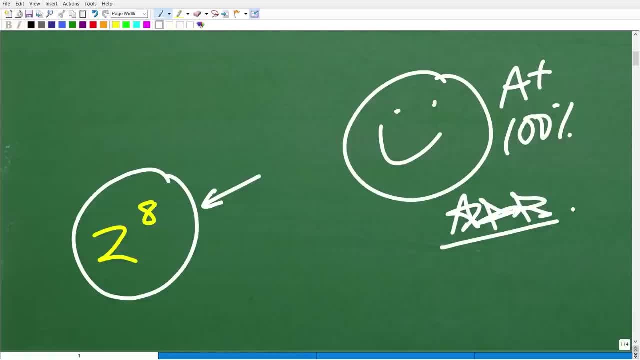 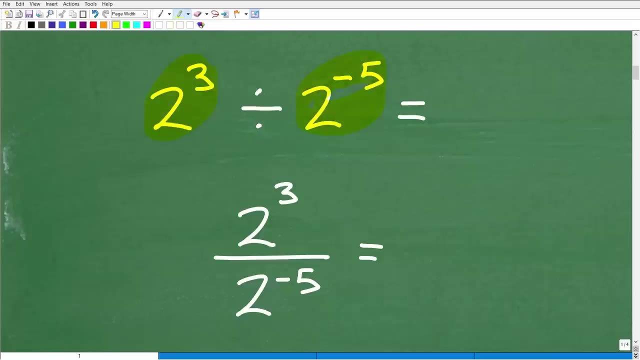 a professional when it comes to dividing powers and exponents. They'll be so impressed with that information. But let's go ahead and get into this right now. Okay, so here is the problem. We have two cubed divided by two to the negative fifth. Now, the way this is written right here is not the best format. Nothing wrong with it, But I want to think of this problem this way. Okay, so this is two cubed divided by two to the negative fifth. 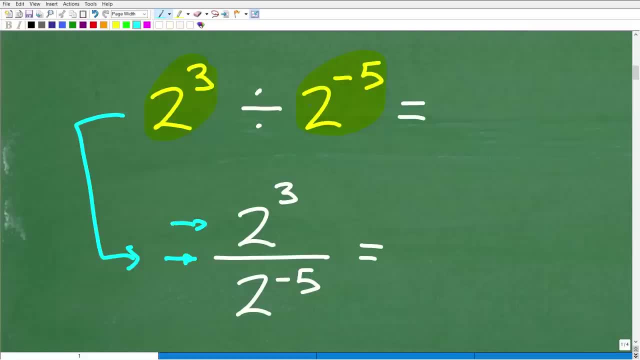 And this is two cubed divided by- I'm going to use this fraction bar here- two to the negative fifth. Okay, so this is the first move that I would make. Now again, some of you could just be like, Oh no, I just knew what to do, And that's great. But let me just suggest one thing here. If you went from this to the correct answer, your teacher might be like: Hmm, you know, did this person really know what they were doing? You know, because you have to show. 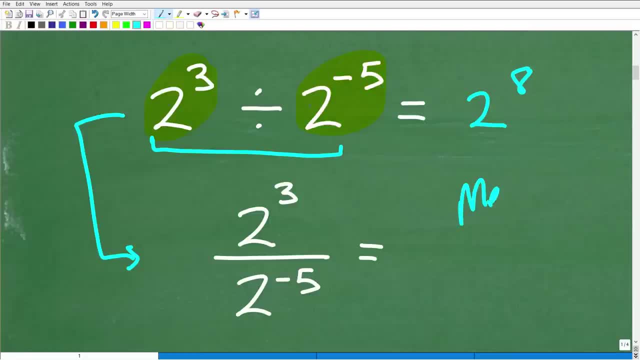 proof, right, And you don't want to do too much, what we call mental math, right, You don't want to do too much steps you know in your brain. Okay, you want to list them out. boom, boom, boom, So your teacher can see, hey, how you're thinking. And two, you can check your work as you go. Right, So you don't want to just take too many steps. You know like, Oh no, I just knew this. My brain is, you know, powerful. I could just tell you the right answer. Well, that's great, And that's fantastic, And you might be able to but list out these steps. So the first thing I'm going to do is I'm going to 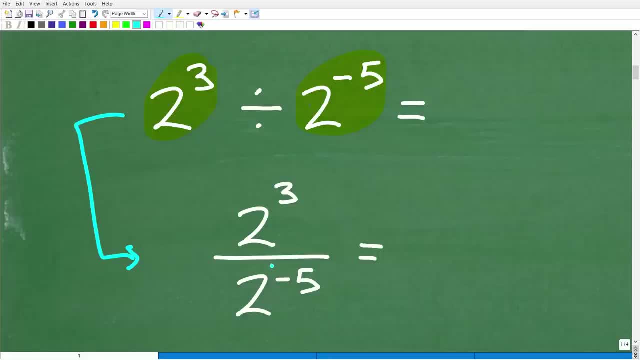 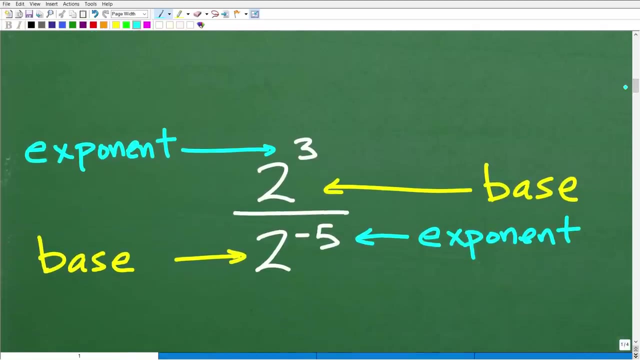 do is write this problem this way. Okay, so that is again the best way, in my opinion- and I've been doing this for quite some time- to structure a problem like this. Now, the second thing we need to know is kind of the language when we're dealing with powers. Okay, So this right here is two to the third power. right, This is two to the negative fifth power. So that's, you know, we're using this word power, But there 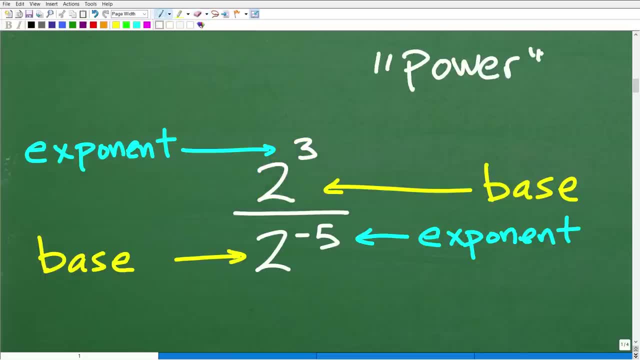 are parts to a power. Okay, now, what are the parts? Well, there's something called the base and exponent. That's what makes up a power. So the big number in a power, this bottom number down here, is the base. Okay, so we can see we have two as a base in this power: in the numerator And the 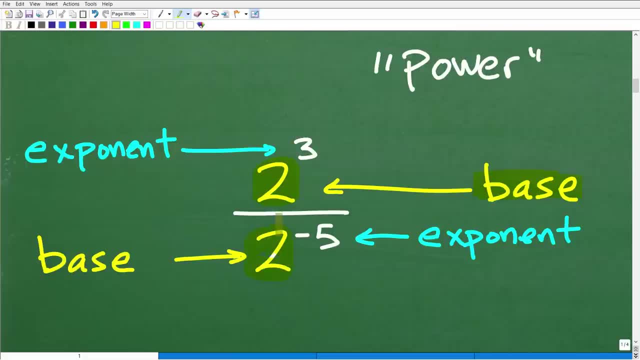 base down here is also two. So this is very important. These powers have the same base. This is extremely important. I'll get back to this in a second. But these small little numbers in the top right are called the exponents. So this down here: two to the negative five. 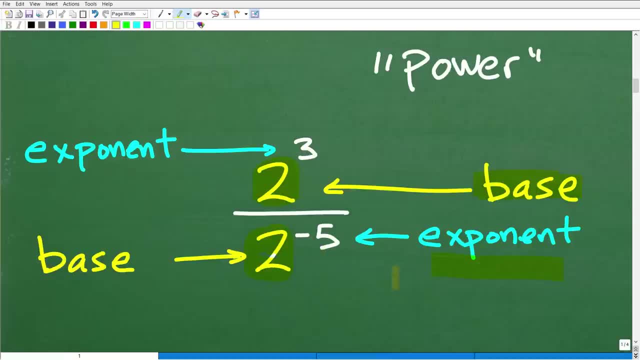 the exponents negative five And up here the exponent is a positive three. But what you really want to focus in on when you're dealing with powers and working with powers is looking at the basis. Okay, So if the powers you're trying to divide, multiply or whatnot, typically the 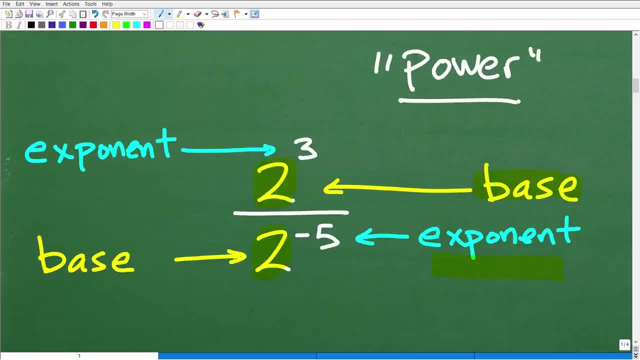 rules of powers or properties- what we call technically properties of powers and exponents- are going to be dependent upon if you have the same base, Okay. so if you have multiple powers, that's great. But, for example, if I have two cubed and three to the fifth, these bases are. 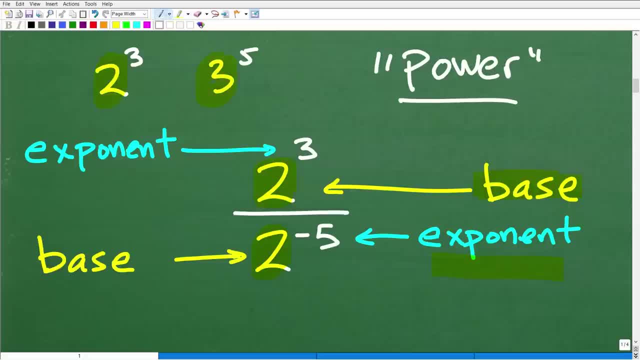 different, So there's really not much I can do with algebraically or mathematically. to simplify the situation, Let's say it's multiplication. nothing I could do, However, once I have the same bases, okay, then I could do stuff. And what can I do? Well, let's go ahead and talk. 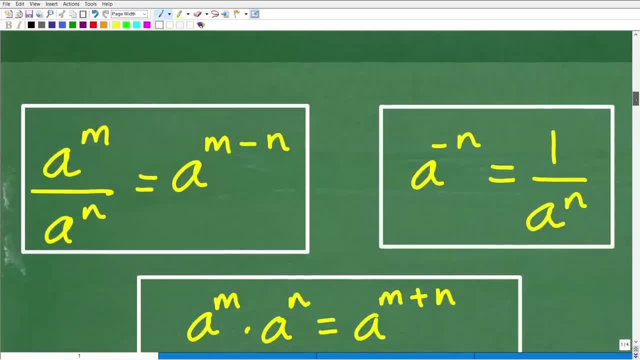 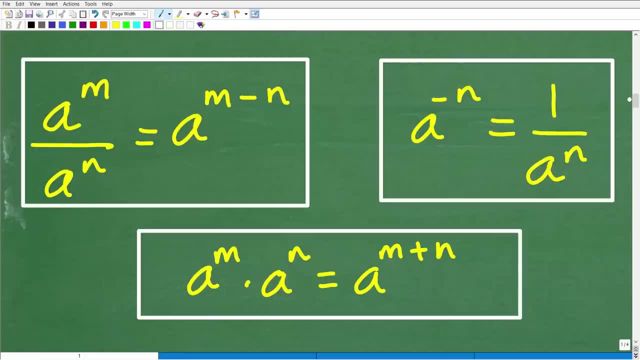 about that right now. All right, So here are some of the rules- not all the rules, but some of the most important rules when it comes to dealing with powers and exponents. So, again, you need to have the same base. So here is one. Now you might look at this and be like: this just looks. 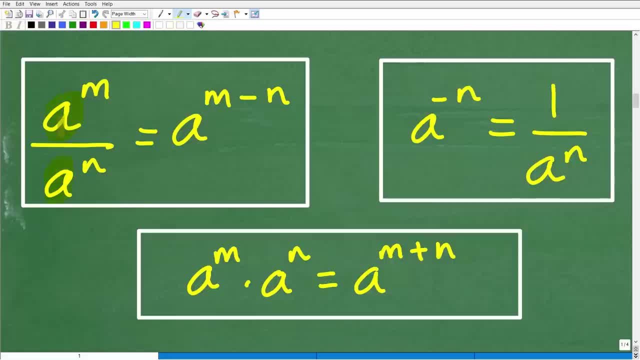 a lot of, like you know, crazy formula stuff. It's not that bad. Okay, So this is. these are two powers: a to the m. this is just a power. a is the base, m is the exponent Down here. a to the n. 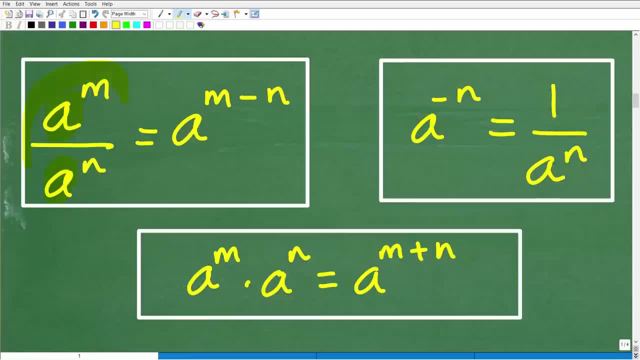 another power. a is the base, n to the exponent. But what's going on here? We're dividing power. This is very much like our situation. Matter of fact, it's exactly like our problem. So when you're dividing two powers with the same base, all we need to do is write that base and find 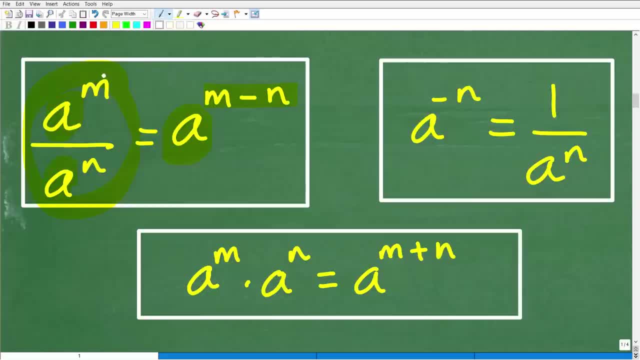 the difference of the exponents. Okay, In other words, we're going to take this m, okay, our numerator exponent, okay, the power that's in the numerator, and then we'll take away the exponent that's in the denominator. So just exactly like this. So this is one way to do this problem Now. 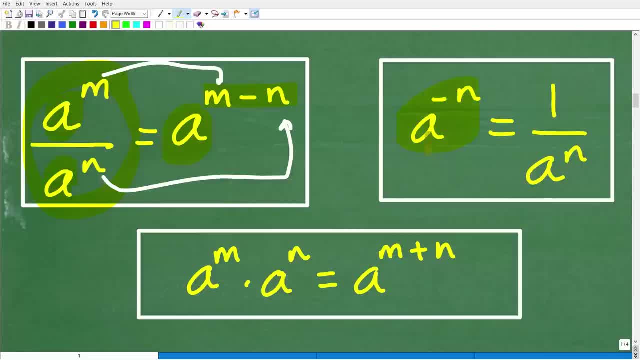 there's another property. This one is often confused. It's negative exponents. A to the negative, n is equal to one over a to the n. I'll explain in a second how this property works. And then another one is this: If we're trying to multiply two powers, 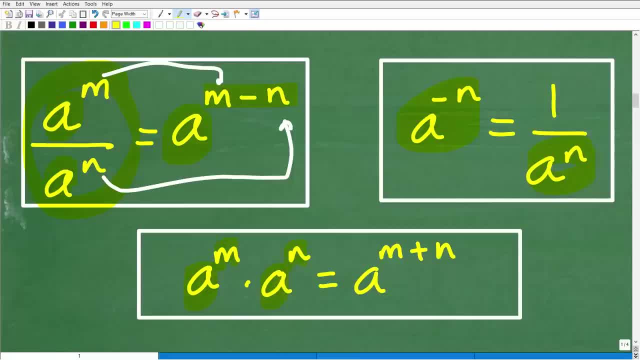 and the bases are the same here- a to the m times, a to the n. what we could do is just write the base and add the exponents, right. So these are three absolute rules that you need to know, And we're going to use these rules in a couple different ways to simplify the problem. But before we do, 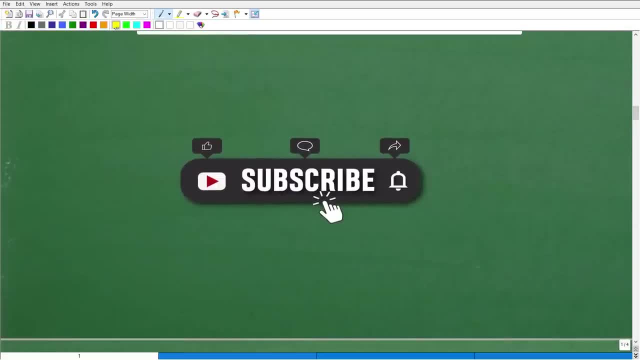 if you have not yet subscribed and if you're thinking about it, just don't think about it anymore. Just hit that subscribe button. You don't even realize how helpful this is for me. Okay, I put a lot of time and effort into my YouTube videos. You know I love to teach from. 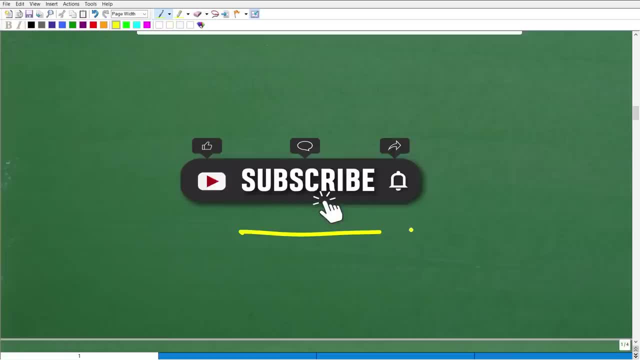 basic math to advanced math, calculus. So you know, by you just clicking that little button- and make sure you hit that notification button to get my latest content, it really really does help. So thank you so much, And now back to the problem. All right, so, as I indicated, we have a. 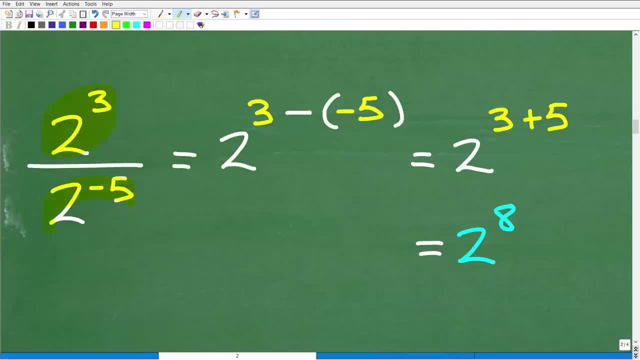 division of power situation where we have this power and we're dividing by this power. Now we these rules here because the bases are the same. we have two here and two here. So the rule is what we're going to subtract the exponents, and this one comes first. okay, the exponent in the 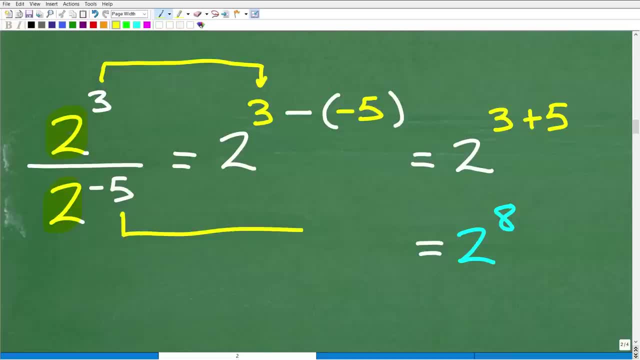 numerator, okay, the power in the numerator, and then this will come second right, And you've got to be very careful with these negative exponents. So this is going to be three minus this negative five. right here, Now let me. let me go back to the rule here, just to make sure you understand what. 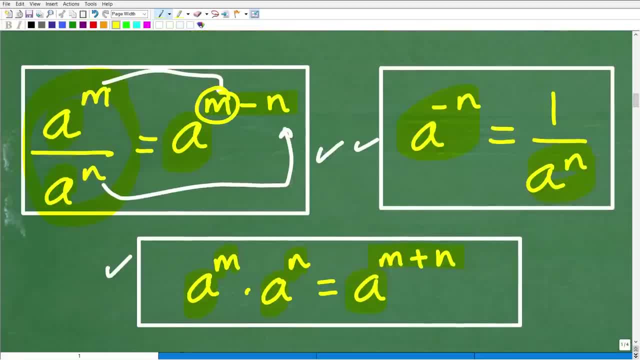 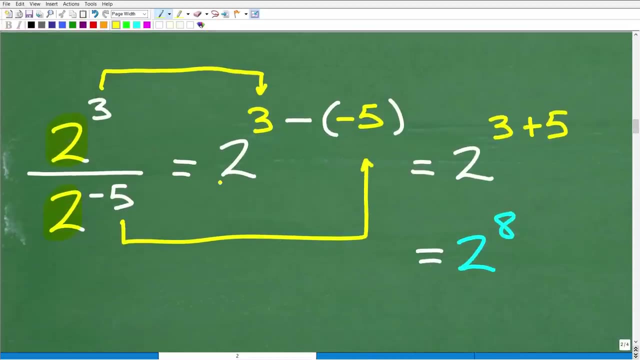 I'm saying So we're dividing power. so it's going to be m, that's the exponent of the power in the numerator, and then n is the exponent of the power in the denominator. you're going to be very careful again working with these negative signs right here. All right, so two cubed divided by two. 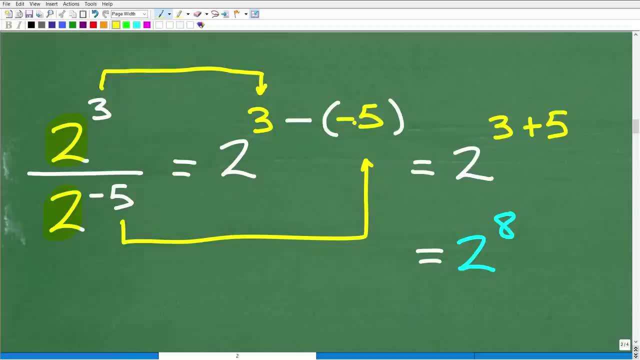 to the negative. fifth is equal to two cubed minus a minus five or a negative five. So opposite, or minus a minus five or negative of a negative five is plus. so this is two to the three plus five. right, All this is equal to three plus five. And the last: 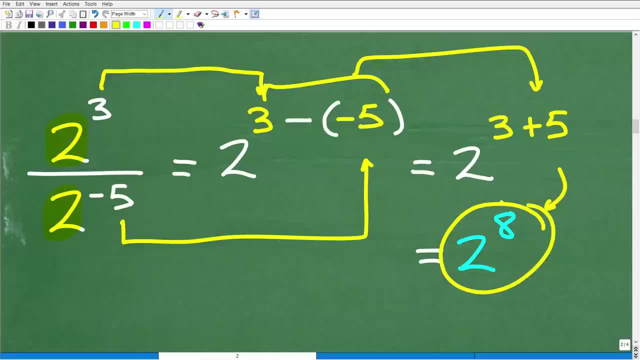 time I checked, three plus five is eight. There you go: two to the eighth power. Okay, so that is one approach to do this problem And I would suspect most of you out there, if you know what you're doing, probably did it this way. But there is other approaches we can take using these properties. 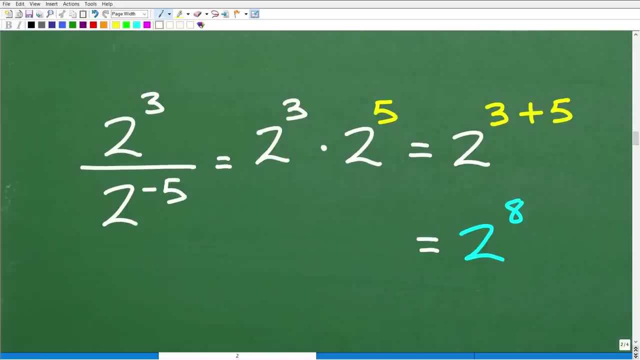 Now, one other approach you could take is we have two cubed divided by two to the negative fifth. I could say to myself: you know what? I'm going to take this power right here, two to the negative fifth and I'm going to move it upstairs. Okay, this is downstairs, is upstairs. Yeah, I know. 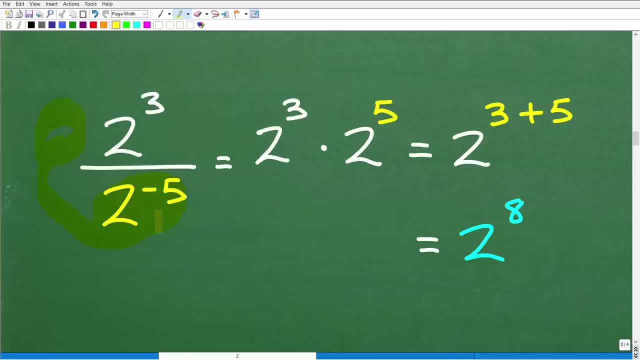 I'm not using proper technical mathematical language, right denominator numerator. I'm just going to move it down from the basement up to the first floor. Okay now, how can I move a power in its current location two to the negative fifth and put it next to this number right here Now? 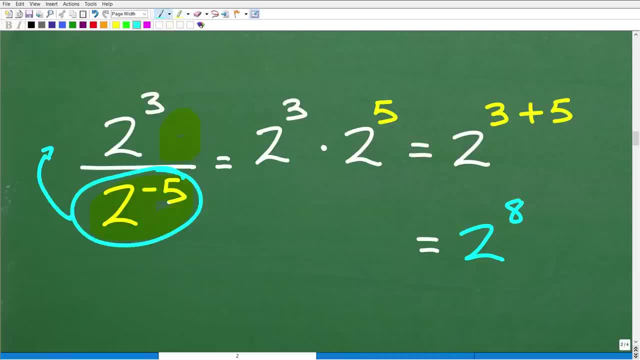 this is actually pretty easy to do. I could take it down to the first floor and I could take it this whole power, and move it next to this number or this power here. all I need to do is change the sign. So, in other words, two to the negative, fifth or two cubed divided by two to the negative. 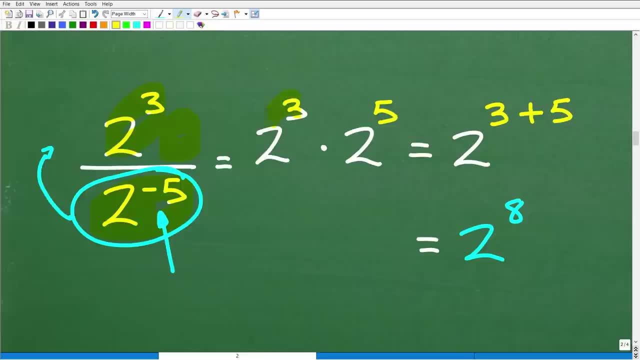 fifth is equal to two cubed- this is my numerator- times two to the positive five. So all you need to do, okay, if you want to move a power from one side of a fraction bar to the other, is simply change the sign. Okay. so this is going to go from two to the negative fifth times two to 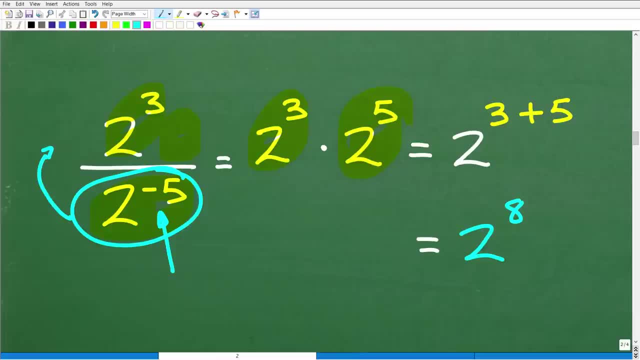 the fifth. Now, this is a very confusing rule And matter of fact, let's just figure this. let me go ahead and just finish the problem here And I'll show you more examples of this. Alright, so we have two cubed over or divided by two to the negative five I'm going to think about, I'm going 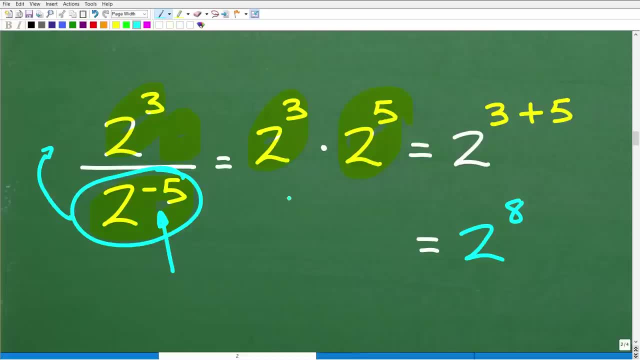 to think of doing this problem as two cubed times two to the positive five. Now, this is multiplication of powers with the same base. Okay, remember, if the bases are the same and it's multiplication, all I have to do is add the. 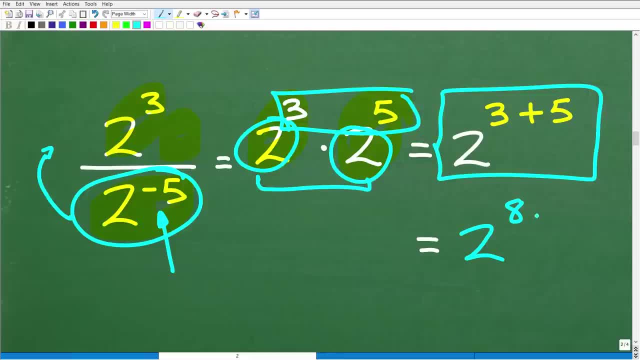 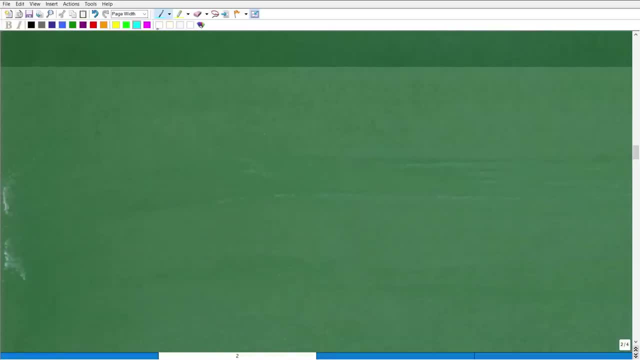 exponents. So this is going to be two to the three plus five. of course, there's our answer: two to the eighth. Now let's go back to this rule right here. I just want to make sure that you understand. Okay, so if I have two to the negative seven over two to the negative nine, it doesn't make a. 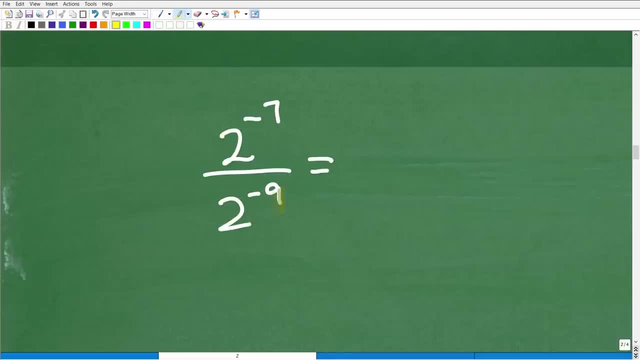 difference. If I want to write these in a different way, I could just flip flop these in all sorts of permutations. So I can take this two to the negative ninth. I can move it upstairs So that becomes two to the positive nine. Okay, so whatever its sign is becomes opposite when you move. 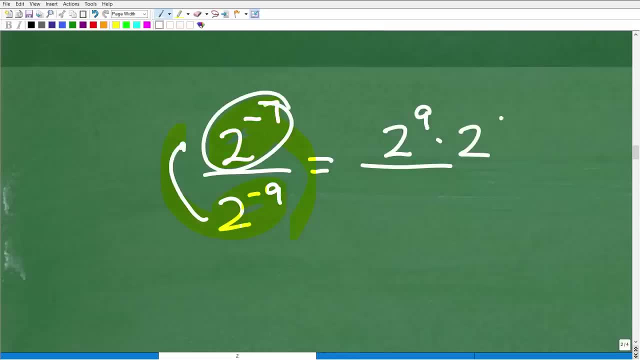 it to the opposite side of the fraction bar. Now I could have this next to my: two to the negative seventh. Or I could say: you know what? I'm going to bring this down to the denominator two to the seventh. Okay, so let's take a look at another example. What if I had one over x to the negative? 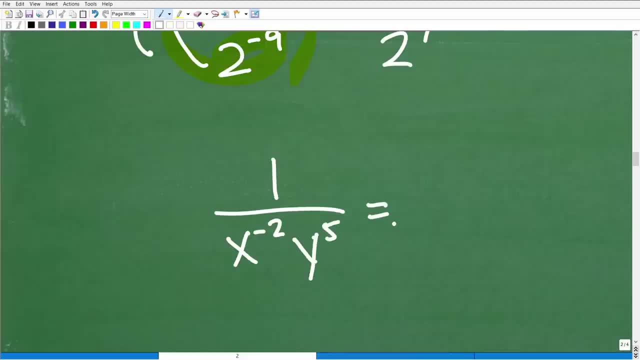 two. use y to the fifth. Okay, well, this works with numbers and variables. I could be like you know what. I'm going to write this this way: I'll bring this x to the negative two, you don't have to do. 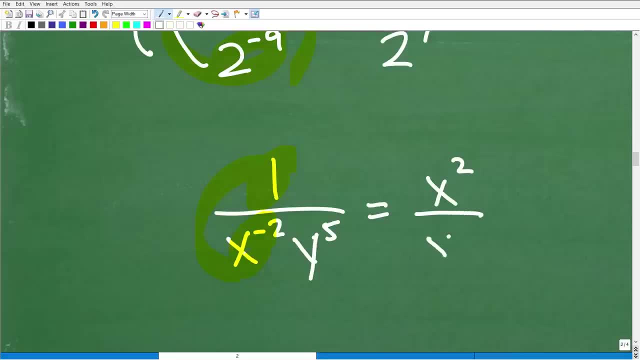 this. it's just something you can do: x squared over x to the fifth. Okay, that's one way of writing it. Another way of writing it: I can be like you know, now, look again, here I'm changing. 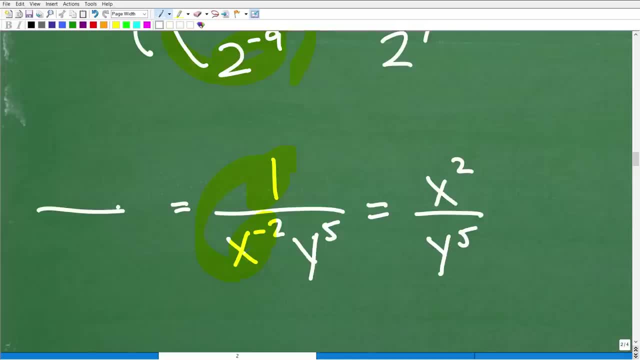 the sign, because I'm moving it to the opposite side of the fraction bar. So I can move this up, So I could have this x squared. and now this positive y to the fifth. I can move that up there and it will just become negative y. 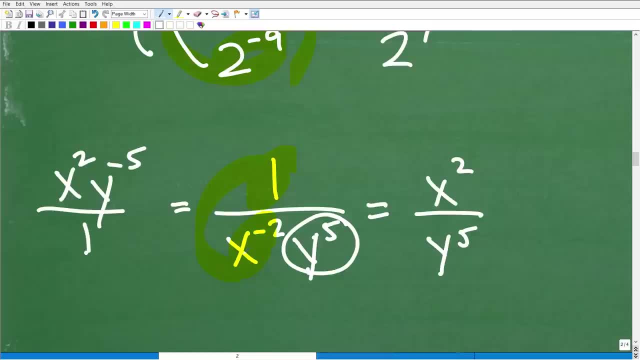 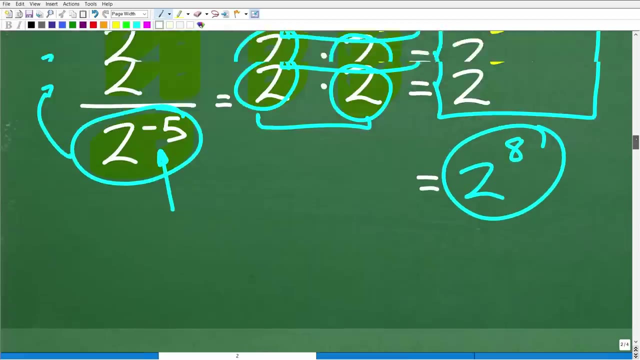 to the negative five all over one, So you can shift powers, their location, where they're at in, in terms of whether in the numerator and denominator. just all you have to do is change the current sign of the exponent. All right, so again you know this is stuff that you're going. 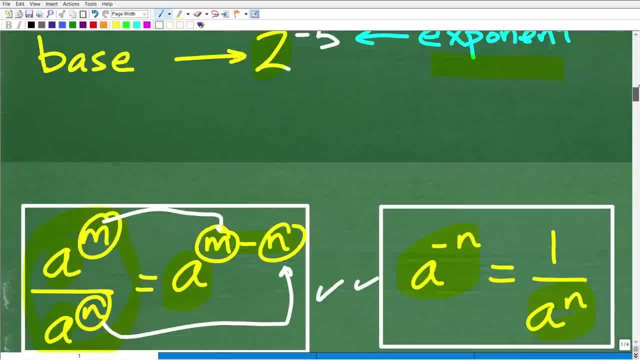 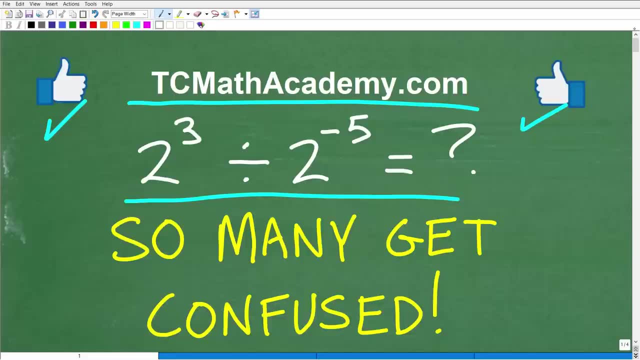 to have to practice very important stuff indeed, especially if you are taking algebra. but again, you know, if you're a little bit confused, that's okay. The only way to get unconfused is to learn you know this stuff correctly and then practice. Okay, it's just.